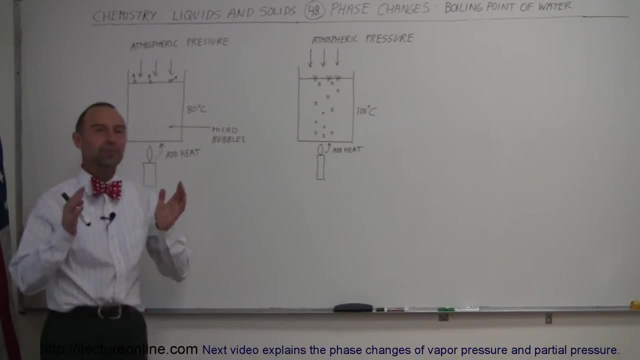 Welcome to iLecture Online, and now we're going to talk about the concept of the boiling point of water. Now it seems very simple: Water reaches temperature of 100 degrees centigrade and it begins to boil. But what exactly is going on? Why does it do that? So let's try to figure it out. 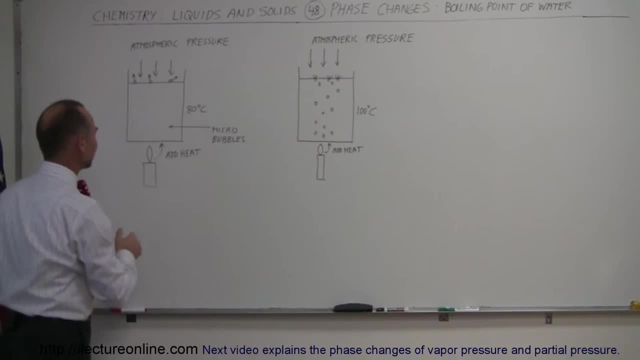 here. So let's say we have a pot of water, It's being heated up. I know it's a primitive heating system, but there is a little candle adding heat to the water And so we're heating up the water molecules that are near the surface here where the heat is being administered. Let's say that. 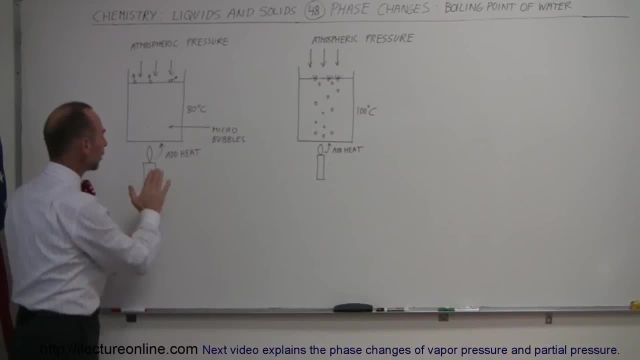 the general temperature of the water here is 80 degrees centigrade, But you know that close to the flame here the water will be hotter and what is going to happen is that as the water gets warmer and warmer, there's going to be some molecules in there that reach such a high. 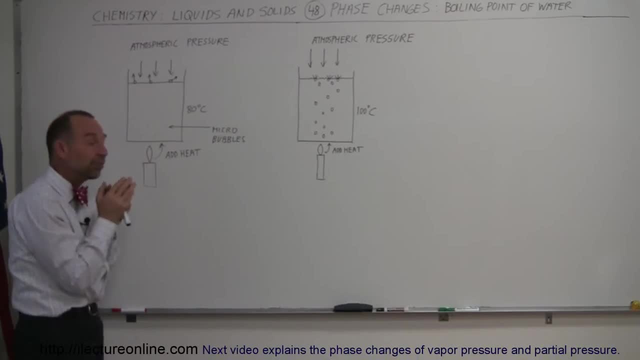 temperature and so much kinetic energy within them that they will actually begin to vaporize right inside the liquid. So what happens then is it creates small, what we call little micro bubbles, Little regions within the water where the water wants to turn into a vapor. However, 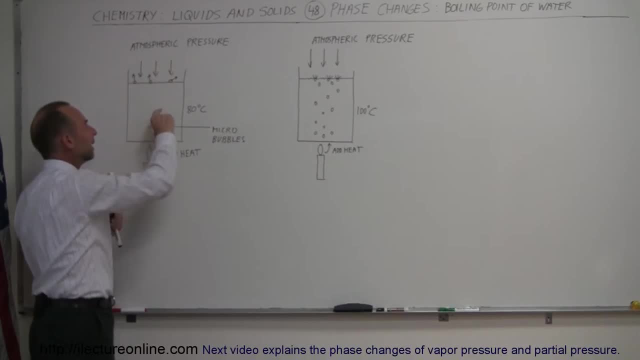 there's a lot of water inside the water, So if I take a little amount of water here, I'm going to an atmospheric pressure pushing down on the water and that causes these little micro bubbles to be squished back down and back down into water. 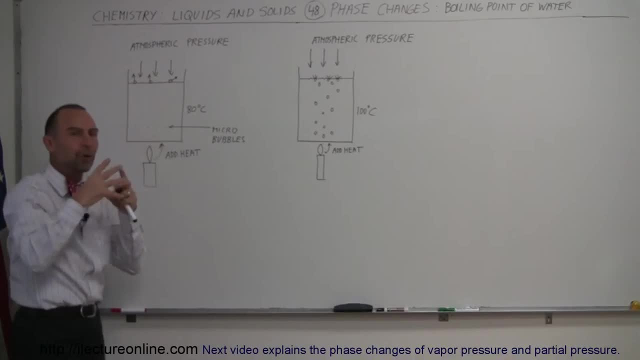 So the atmospheric pressure doesn't really allow these bubbles to really form and blossom. Anytime a few molecules try to form a micro bubble, atmospheric pressure squishes it back down and so that prevents the water from beginning to boil. So the heat simply just gets distributed within the water and slowly the temperature of water 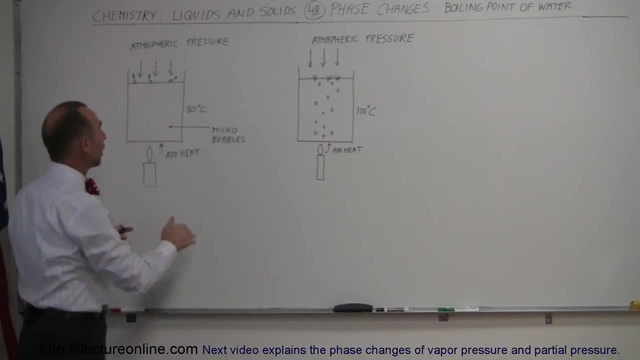 continues to increase at 81,, 82,, 83 degrees and so forth. Of course, at all times you'll still have what we would call evaporation, The molecules near the very top. they do have, at times, enough kinetic energy to jump free. 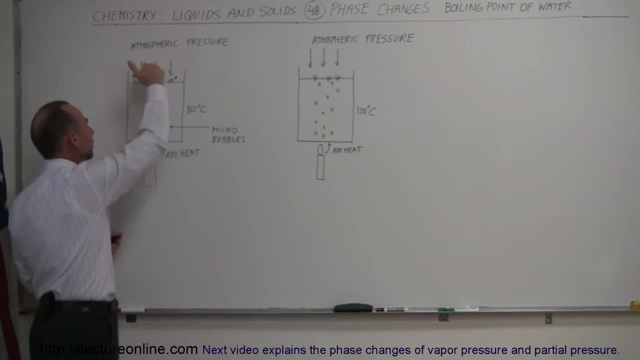 from the cohesive bonds of the other molecules, and of course there will be condensation at the same time, But at very high temperatures definitely, the rate of evaporation will far exceed the rate of condensation, and so water molecules will evaporate, but the water will not be boiling. 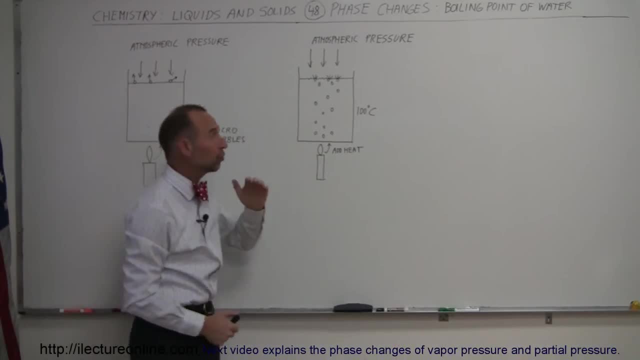 What happens now? when finally the water reaches 100 degrees centigrade- assuming that outside it is outside Atmospheric pressure? What happens now is those little micro bubbles. they begin to grow So much heat is being added to the water that once the water container, all the water within. 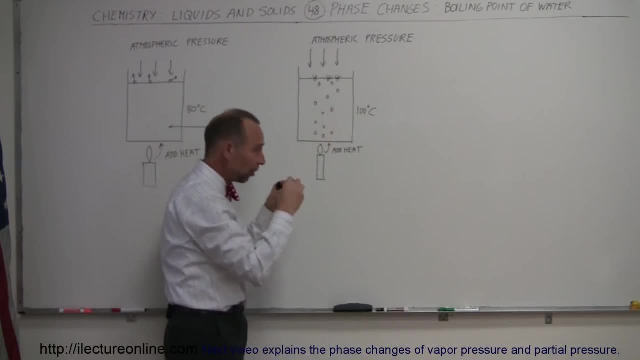 the container now reaches 100 degrees centigrade, any additional heat being added to the water is not used to increase the temperature of the water, but is now used to turn the water into vapor, because at that point, when the water reaches 100 degrees centigrade, they 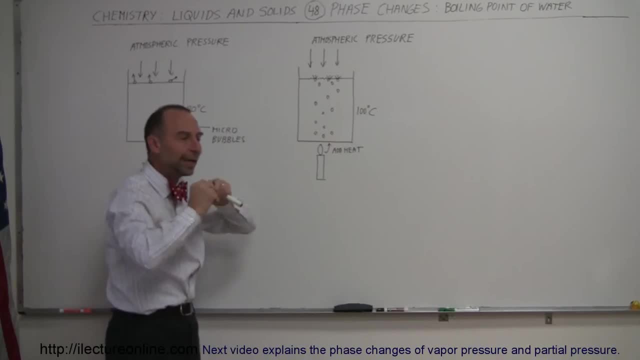 have so much kinetic energy that they will actually push each other away and turn into little bubbles of vapor. and you can start seeing all the bubbles of vapor to start in the water, because the water molecules are so energetic at 100 degrees centigrade that they actually will turn into vapor with any additional heat given to them. 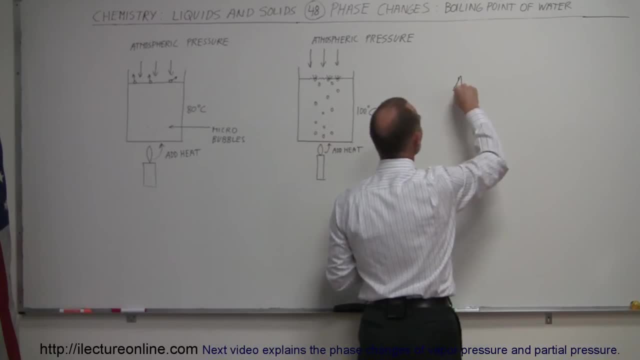 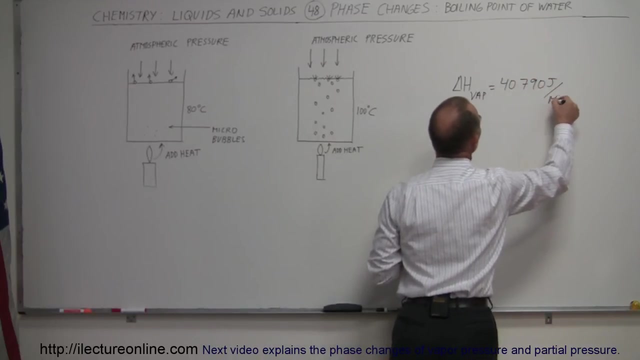 Of course it does take energy, The enthalpy of evaporation of vapor- I should say vaporization, that's a better way to say it. the delta H for vaporization is equal to 40,780.. Okay, 40,790 joules per mole. 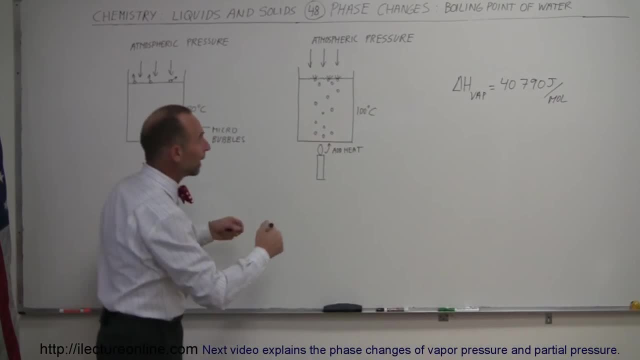 So before an entire mole of water molecules turns to vapor, you will have to add 40,790 joules, So the rate at which water is being vaporized in this matter- because boiling is a form of vaporization at a high speed- it all depends upon how fast you can put that extra heat. 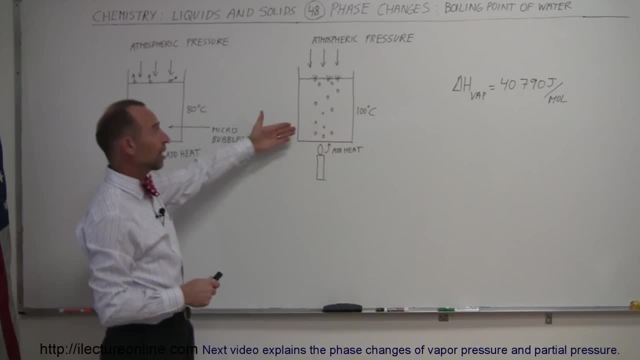 into the water. So let's say that every minute you can put 40,790 joules of energy into the water. then every minute you would turn one mole of water into vapor And that vapor then would escape out the pot and you could then slowly see the water. 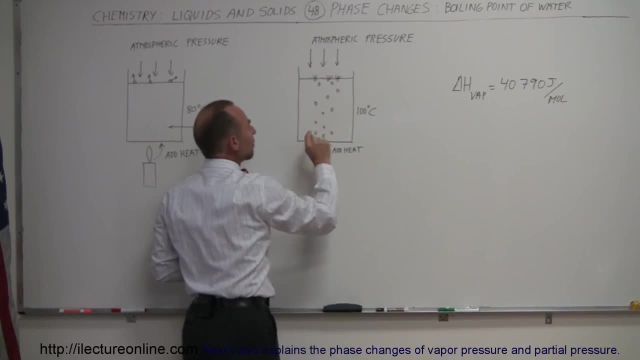 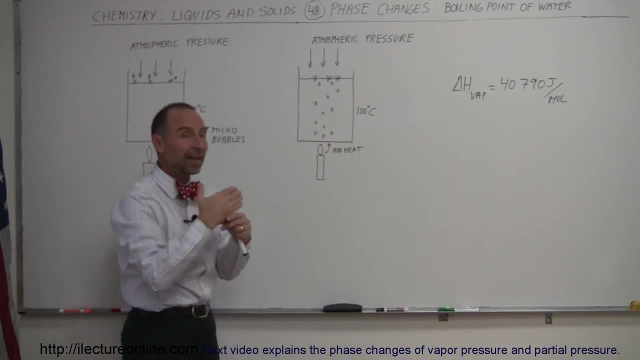 molecule drop. So since the pressure inside here is now equal to the atmospheric pressure- because that's what happened- the vapor pressure can be the same as atmospheric pressure at 100 degrees centigrade. the atmospheric pressure can no longer squish the bubbles and the bubbles. 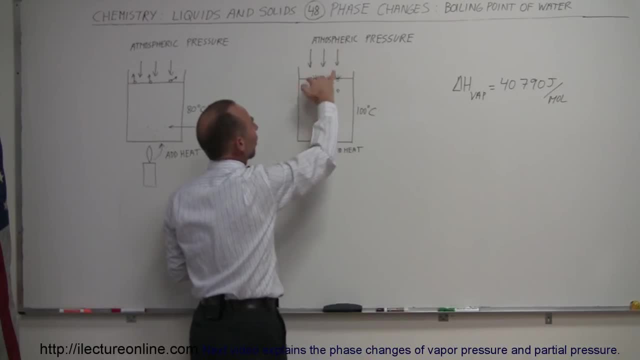